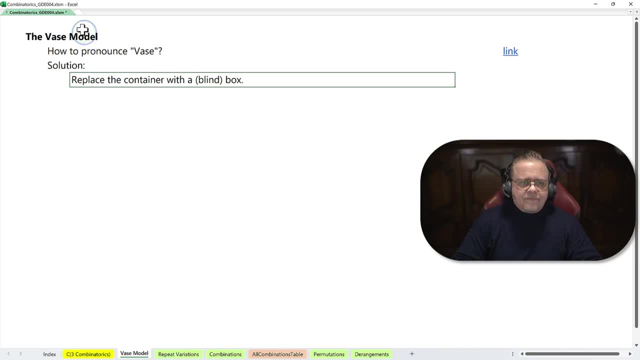 going to replace the container with a box. Voila, there it is, The box model, officially called the VAS or VASE model. What is it? Well, it's a blind box. We don't want to look inside and we want to keep an element of. 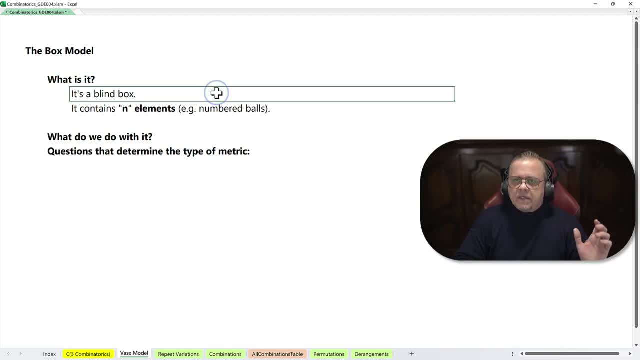 randomness involved here and we put inside that blind box n elements. Think of them as numbered balls n elements. What do we do with it? Well, we pick balls from the box, one at a time and in a sequence we perform k amount of. 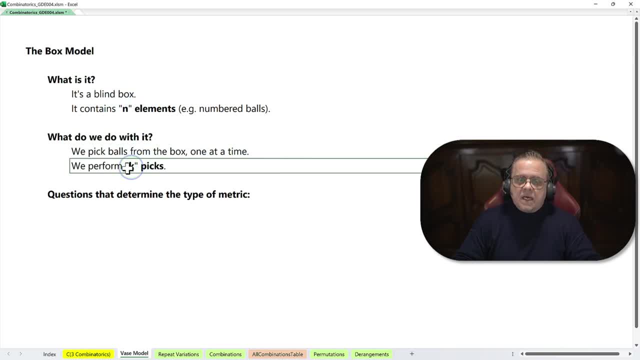 picks. So it's a general case: n elements and we pick them k by k. In order to determine the exact metric, we need to answer a few questions. Two questions are very common here. The first question is: do we return the ball to the box after each individual pick, Yes or no? If we do, we 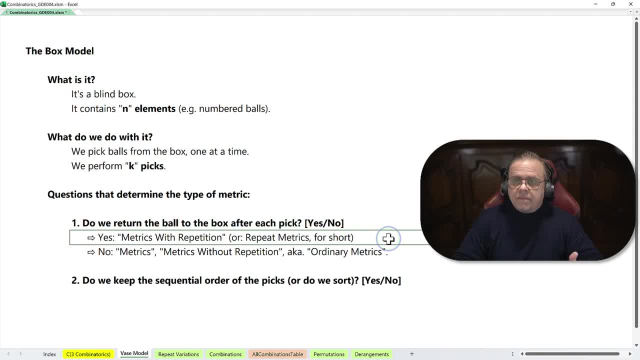 talk about a metric with repetition, or a repeat metric for short. If we don't, we just call it the name of the metric, or you could call it the ordinary metric. In any event, it is the metric without repetition. The question we need to ask ourselves is: do we keep the sequential order of the picks? 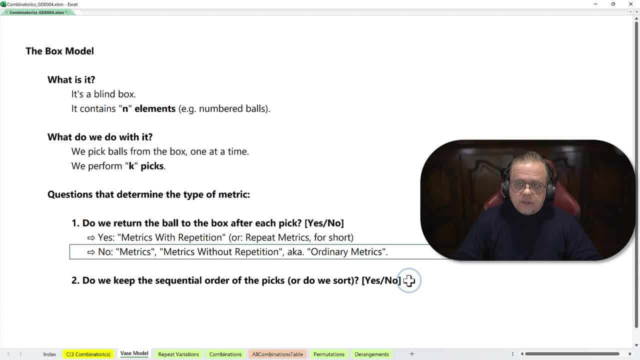 or not, And in the second case we could sort the numbers. So if we keep the sequential order, we talk about a variation. If you apply a few more restrictions, we get permutations. Yeah, if we sort the sequence, so we don't keep. 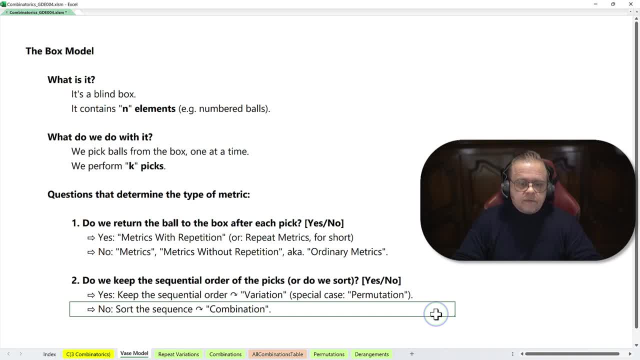 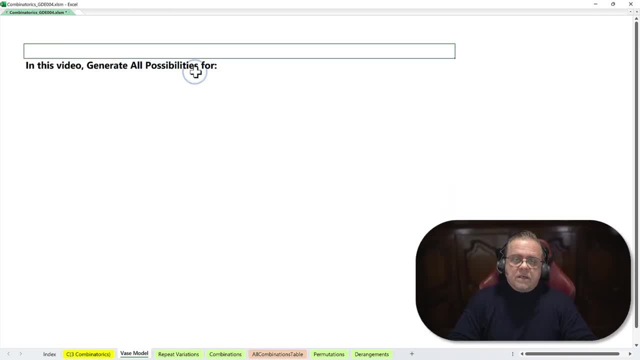 the sequential order. we talk about a combination. What are we going to do in this video? We're going to generate all possibilities for these metrics: repeat, variations, combinations, permutations and, as a bonus, derangements. The latter here, I will define when we get there. 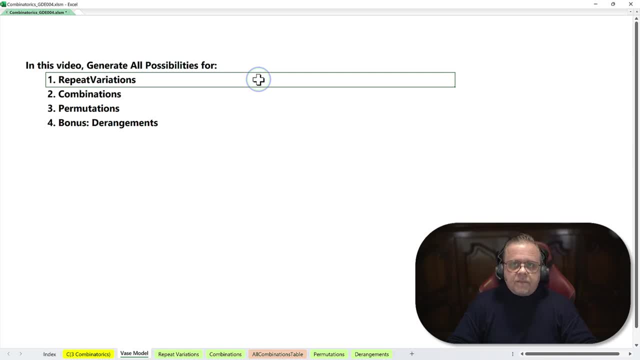 By the way, repeat variations, or variations with repetition as mathematics calls them. in Excel they are called permutations with repetition, but technically that is not the right term, So I'm going to keep the term repeat variations. If you think those are the most abstract things we're going to encounter today, we never use. 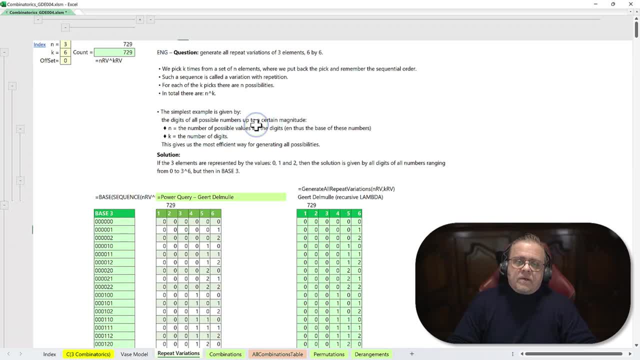 them in real life. well, you'd be wrong, Because for repeat variations the most simple of all examples are the numbers we use on a daily basis, the digits of all possible numbers up to a certain magnitude, where n the number of elements here is just the number of possible. 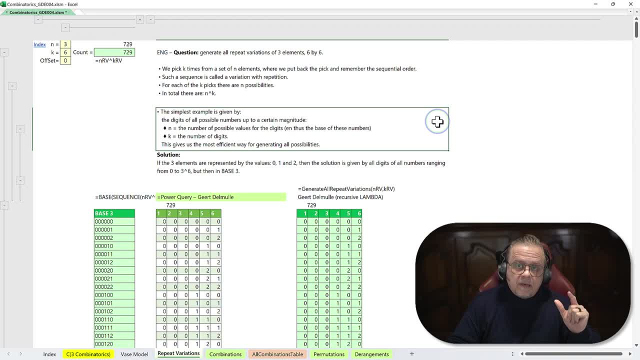 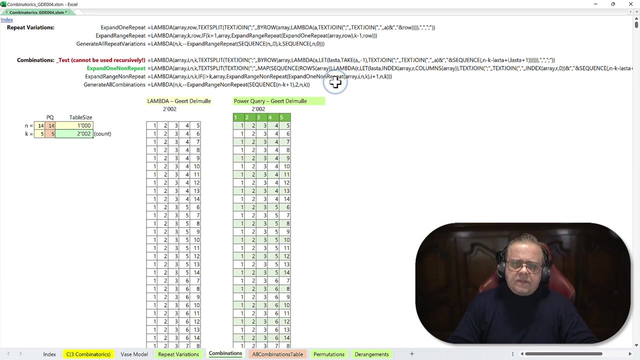 values for the digits. In mathematics we call that the base, And k- the number of picks- is the number of digits itself. So we can easily take that into account. it helps us to generate those repeat variations For combinations. well, we can do that. you can use some lambdas, but they are quite inefficient. 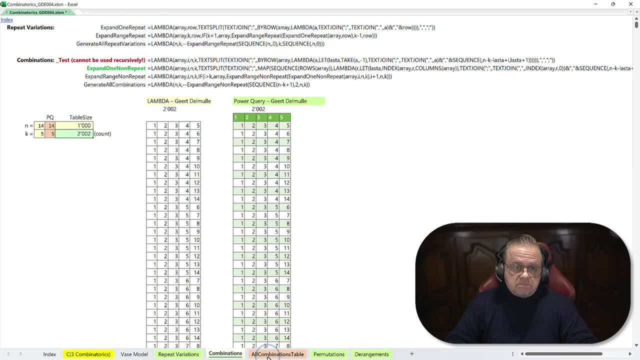 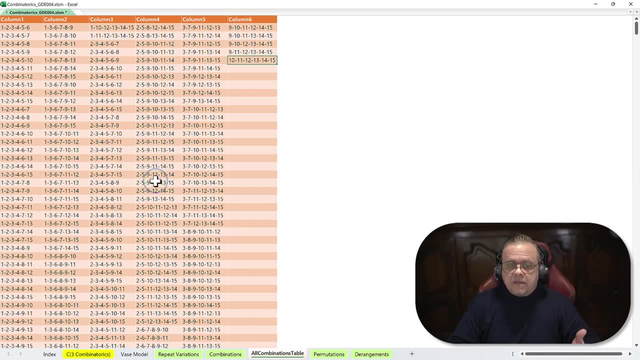 at least mine are, Be it recursive. Hmm, You can do it and you can sort a table a little bit like this, and you can look at these nice combinations and derive the necessary rules that you need to apply in order to generate them. 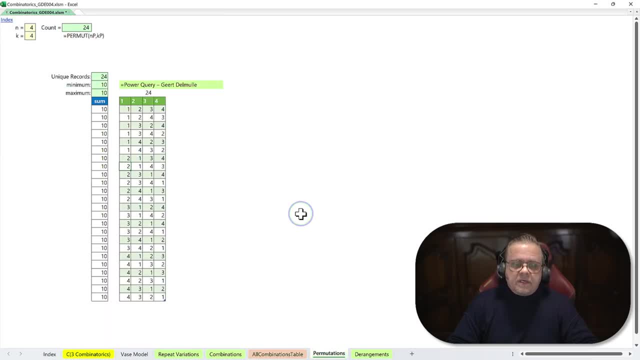 That's what I did, And we have permutations here and finally, the derangements as well. Now, technically, we haven't written those power query functions yet. so you know what? Let's get to a new workbook And start writing those functions from scratch. 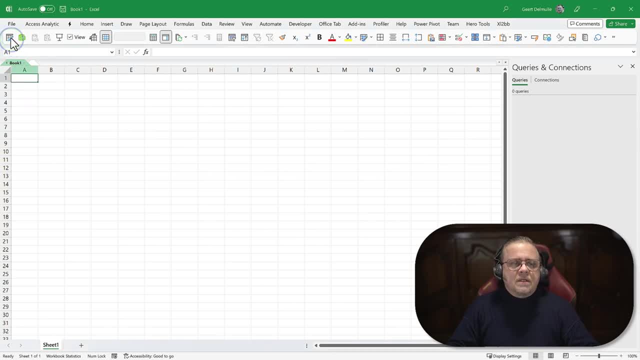 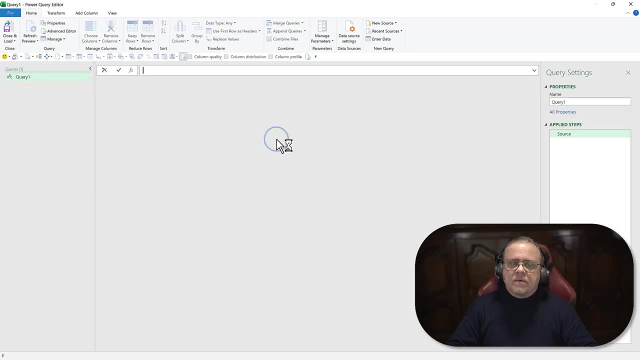 Okay, here we are in a new workbook. Let's open up power query. In power query, let's start a new blank query And I'm going to give it a name: generate all templates. I'm going to create a generic template first. I will reuse a template for all the subsequent. 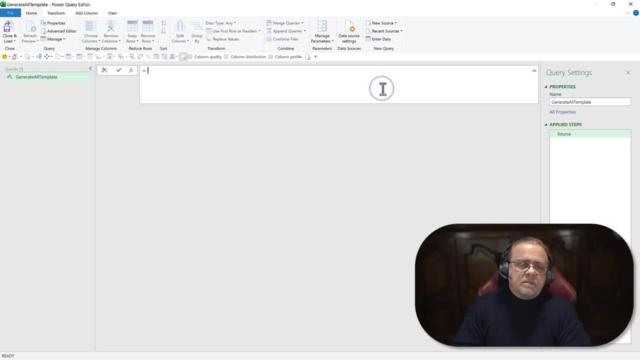 functions. It is called determiner playing music. That makes it most efficient. Alright, so N as a number, general case, K as a number results as a table goes to. The main function we're going to use is called this list of accumulate, right there. 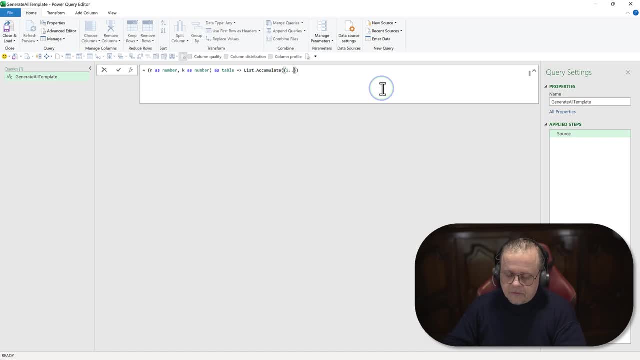 We're going to iterate over the columns to do that? Yeah, All right, So you understand the theory of Bernoulli to K. why do we start from column number two? because the first column is going to be seeded. the seed it's going to be table from columns, plenty of curly. 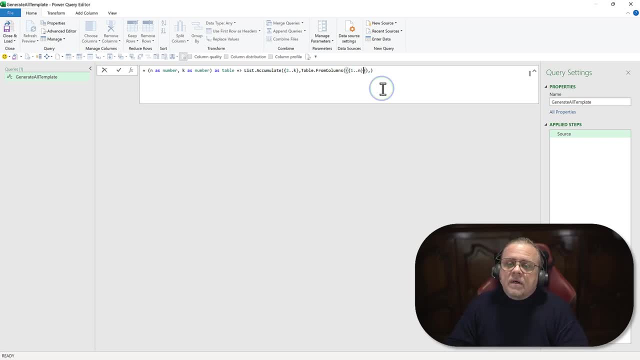 brackets: one, two, n, and we're going to call it column number one. that's the seed completed, right, of course, our custom function. it's like always a little bit the same state goes to state, an index goes to what. all right, here we're going to build our field formula. I need a double function. but before I 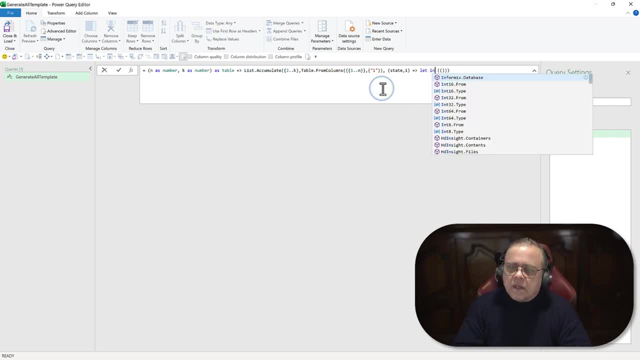 started function. I need a local variable, just a small one. I'm going to call it header, and it's actually the text from I, which is just I in text format. then they reuse it a few times first function. what we're going to do is add a column. 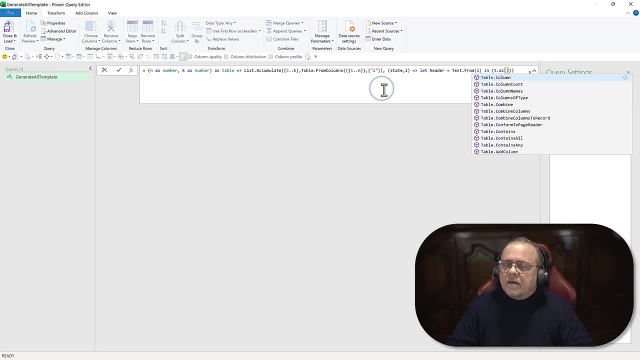 table add column. right here at the bottom I'm going to add state column, whatever is in the header, and we're going to say each same list as in the seed and that's table dot add column done. the next function that we're going to wrap here needs the header variable as well and it starts there and it's. 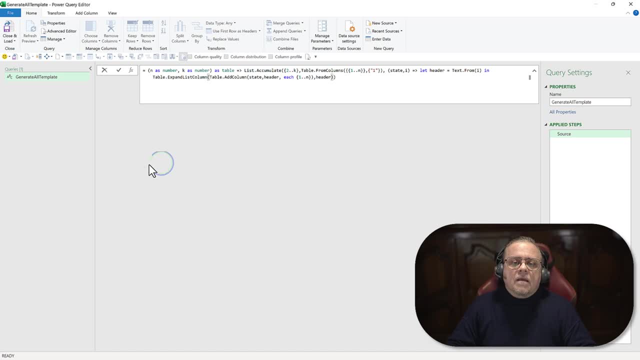 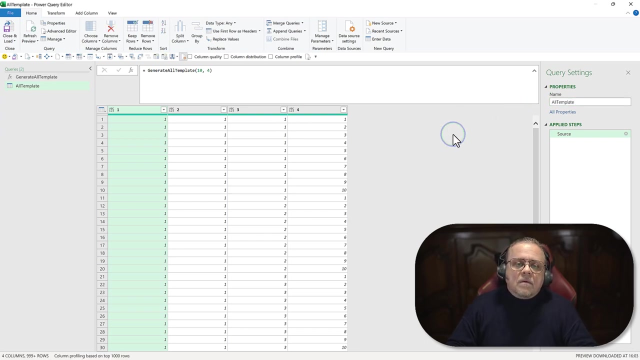 table dot. expand this column. and that's the template done. let's test it and give it a name right there. as a matter of fact, all template is already a useful function. it's actually the repeat variations function, yeah, but it starts from one which is rather unusual. let's amend that and generalize. 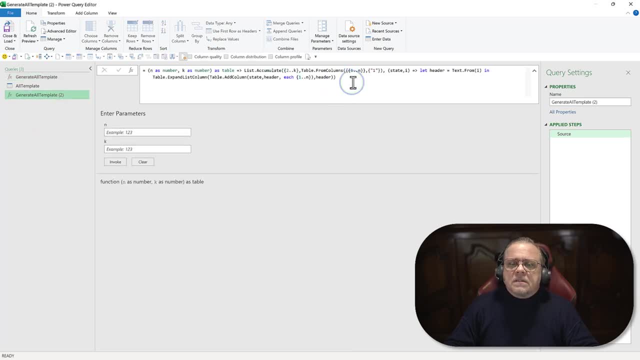 it kind of duplicate the template. of course we're gonna start from zero, so we shift everything down, just like in power query, zero based voila. and then what I'm going to do here is generalize it a little bit: offset right plus the offset quickly. if you want, you can do that all the time, I'm only gonna do it here. got three. 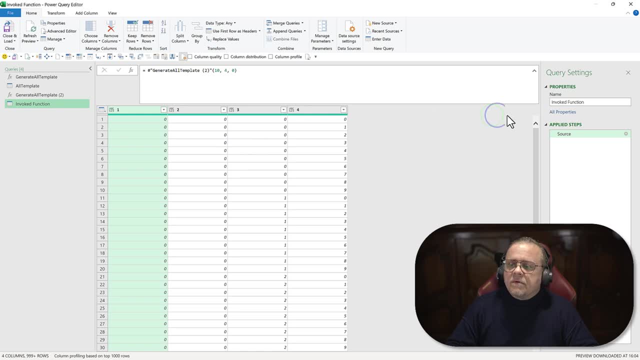 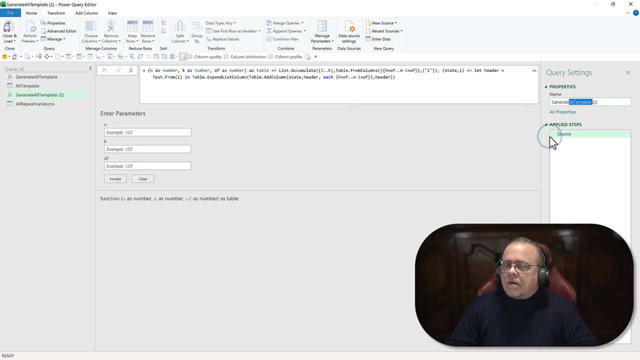 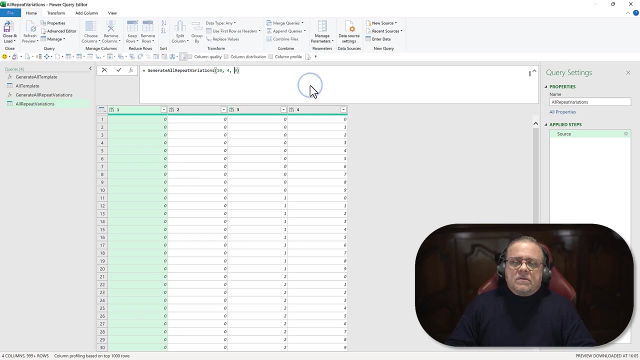 things: three parameters. let's invoke it right away, that offsets can disappear. all repeat variations is what we're gonna call it, and frankly, it's a little bit of a pain in the ass, so I'm gonna put that there as well. okay, let's have a look. so this is the general case for repeat variations. it's the way we write. 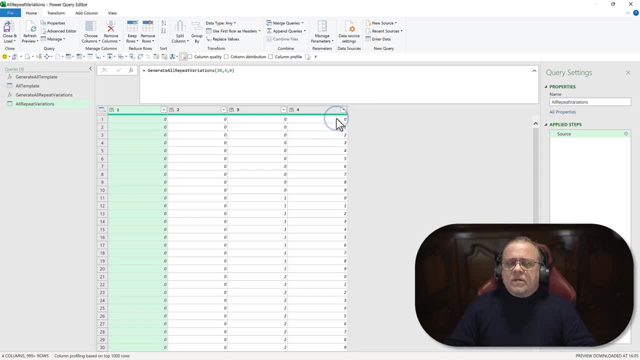 our large numbers, of course, using various digits. we start numbering from zero on the right side, increment all the way up to the number of elements, which in this case is called the base minus one. then we roll over to the second digit and keep incrementing. we all know how the large numbers works, right. fine, you can do like. 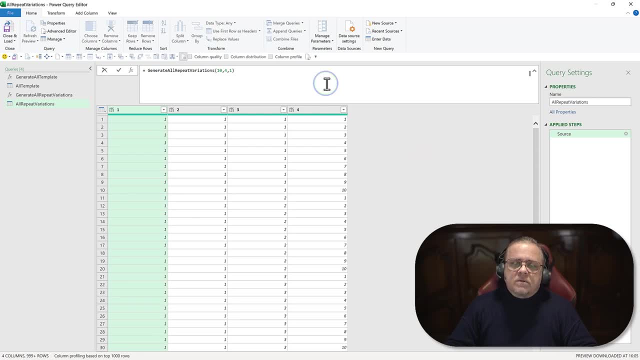 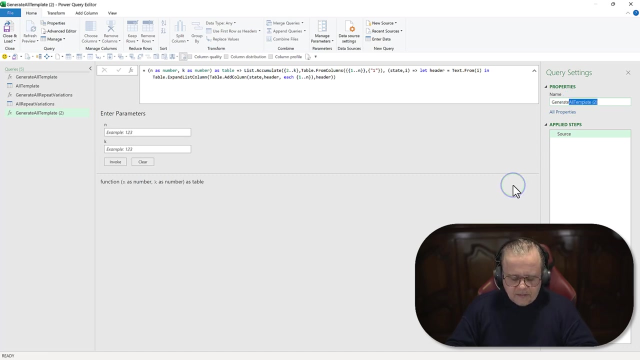 this: starting from zero, starting from one, starting from whatever you like, and that's that. the offset is a small complication. I will not add it to the subsequent functions. all repeat variations done, fine, next up, let's do combinations. start from our template again, right, let's give it a proper name. all combinations. what do we need to do? how do we need to amend? 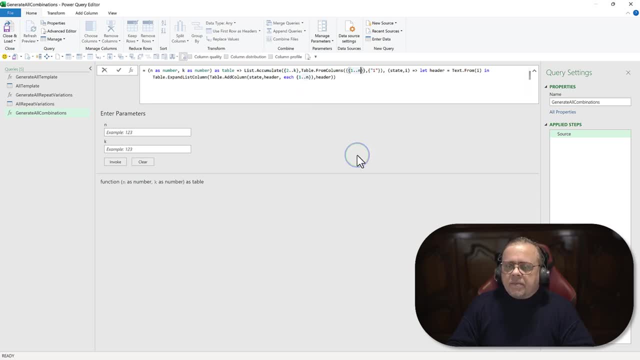 this function well. we need to amend it on a couple of places. just the lists, but that's it. here I need to put as an upper limit n minus k plus one which generalizes in the field function to n minus k plus i and the lower boundary here in the seed one is okay, but in the field formula it. 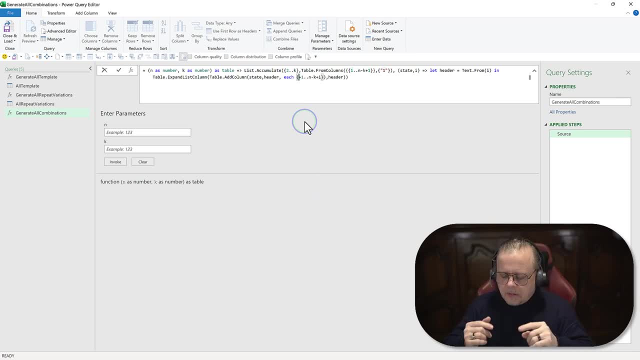 is whatever is in the previous column plus one. how do we do the previous column? well, we take the entire record, we say, hmm, a record to list, and then we say list dot last, and this is all combinations done. this is how we refer to mom: whatever it is in the last column, remember that we're gonna. we're gonna reuse that entire. 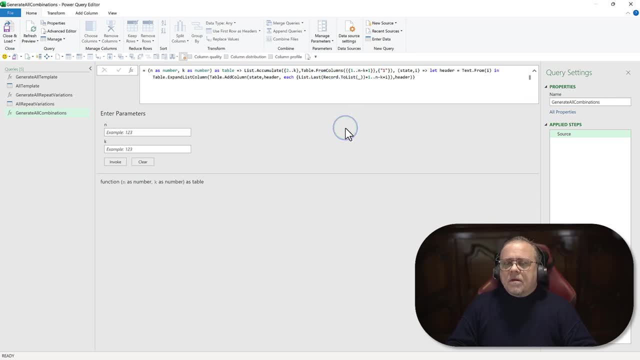 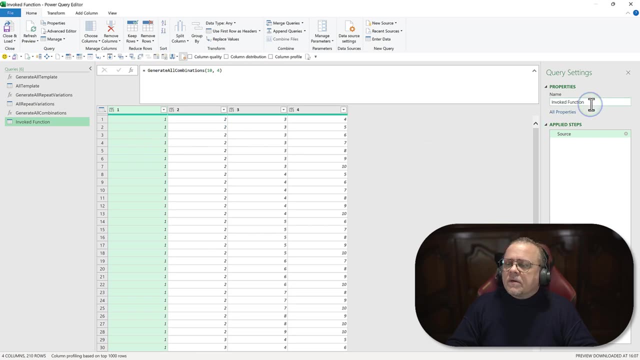 function shortly. this is all combinations done. let's go and check it out. we're gonna rename the application so we have ten, four by four, two hundred and ten rows, which is correct, and it starts in the first record as one, two, three, four and it will end into seven, eight, nine, ten. yeah, that looks alright. this is all combinations done. 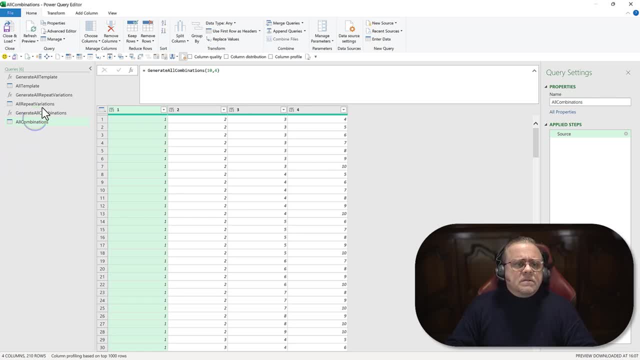 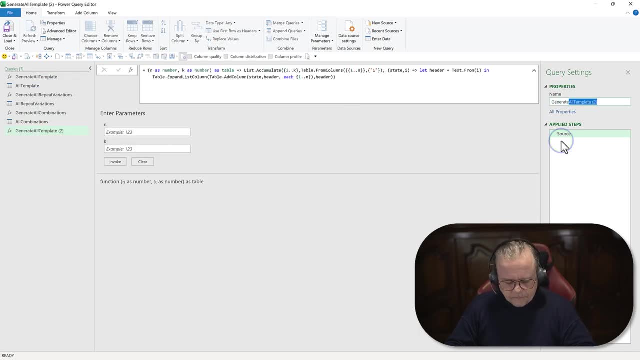 next, all permutations. let's recycle our template, give it a good name: all permutations. how do we need to amend? well, the seed is the generic list of full lists. that is good. but the field formula- we're going to amend it in such a way that we remove duplication. that 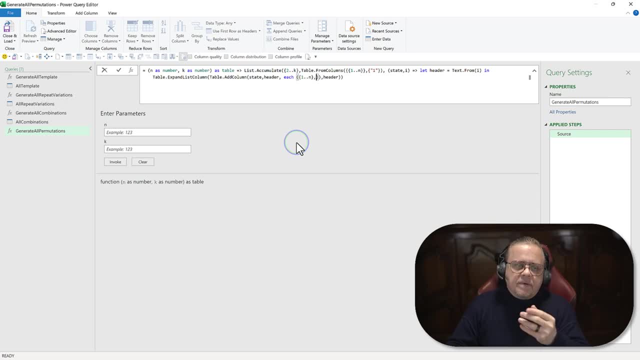 we remove repetition, because it's ordinary permutations here. all right, so we need to remove whatever exists already. uh, oh, yeah. well, we know how to do that. we're going to add some list. if we're going to wait, let's write list. we want to have our. 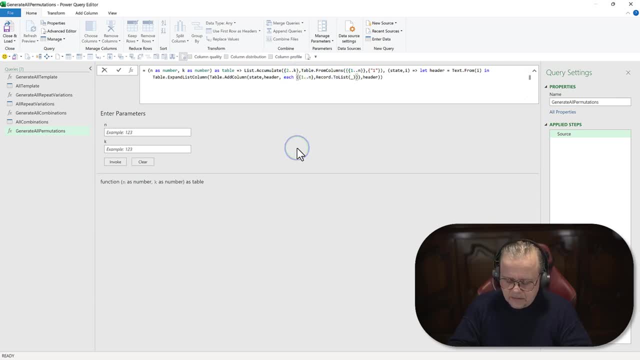 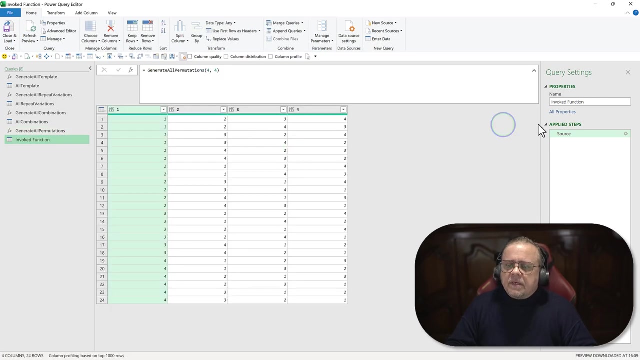 list grow to what we represent. so let's write this here real quick. we wonder, came out right? so list of full lists is one, two, three, seven, eight- completa list, yes, and that we want to not affect, or Douglas, okay, what do you mean? byide, give me if I confuse something. 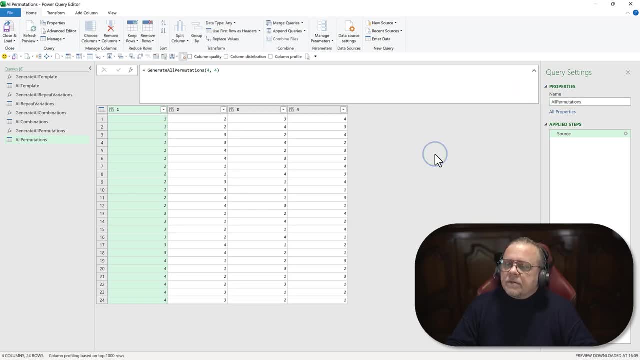 this, make it two or three. We need to be in the right place to stop That. nextier thing: permutations. Fine, So for 4x4, we got 24 records in total. It starts with 1,, 2,, 3,, 4, and it ends 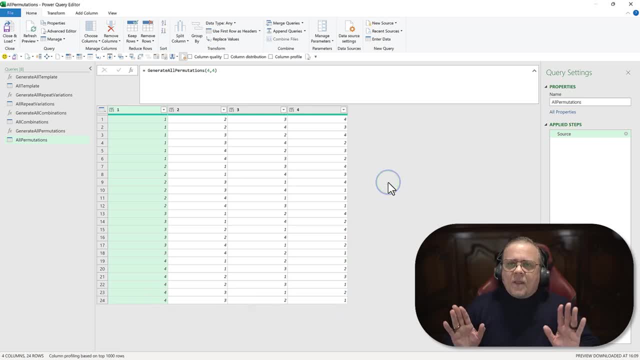 in 4,, 3,, 2, 1.. Beautiful, All permutations done. As a little bonus, let's do another one, and they're called derangements. All right, I'm going to start from permutations, because derangements 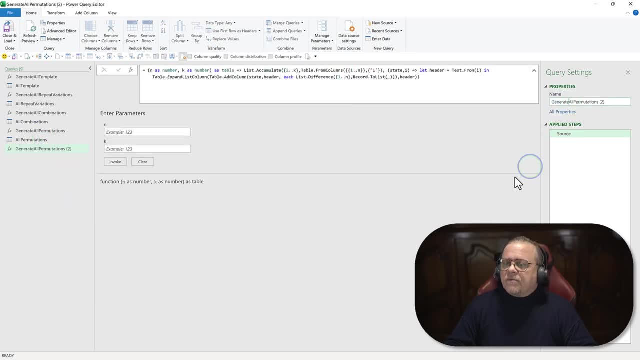 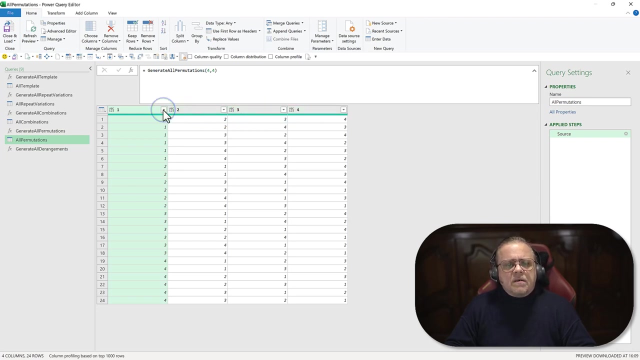 are actually a special case of permutations. Let's rename it and I'll explain it immediately. If I go and look at all permutations, a special case for derangements is that the original position must change, meaning element number 1 cannot go to column. 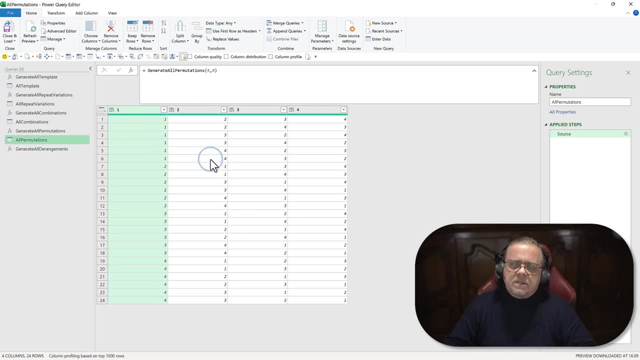 number 1, element number 2 cannot go to column number 2, etc. All permutations are special cases of permutations. All elements in the original position need to be displaced, deranged. It's a thing. I'm not making this up, This is no joke. It's not so difficult, but it's not a joke, All right. 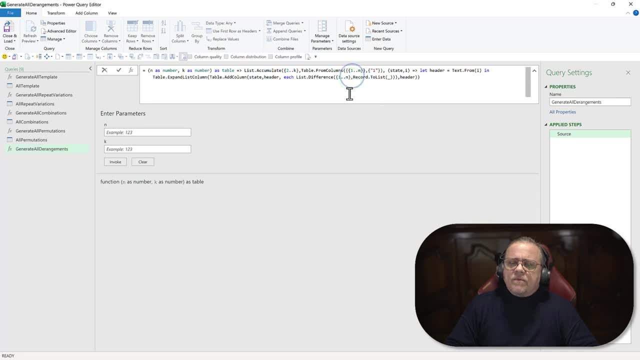 so how do we amend this formula here? Well, first off, the first column needs to start from 2, not from 1, because that is prohibited. Next, we need to remove a little bit more than just the current record. We need to remove the current record and make sure that the running. 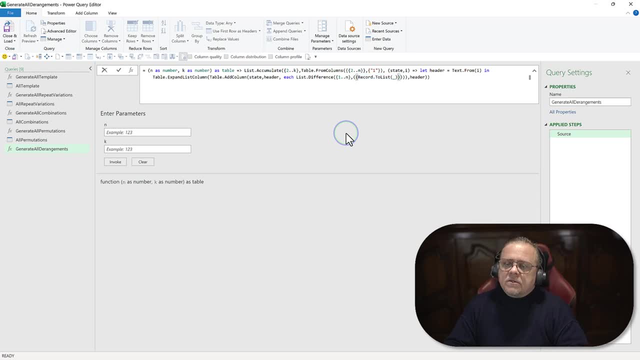 index i is not present either. So what do we do? We add a second list containing i and we combine that with the current record using listunion and that complete thing gets removed using listdifference from the complete list. This is all derangements done. 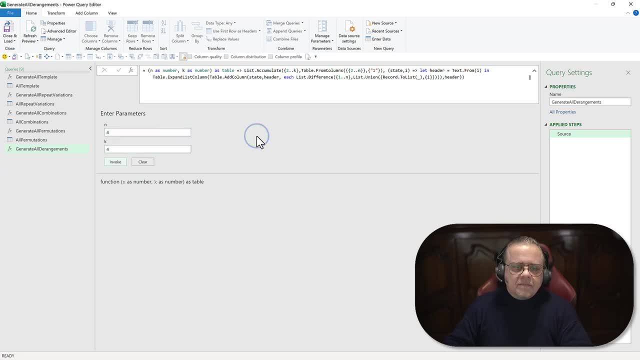 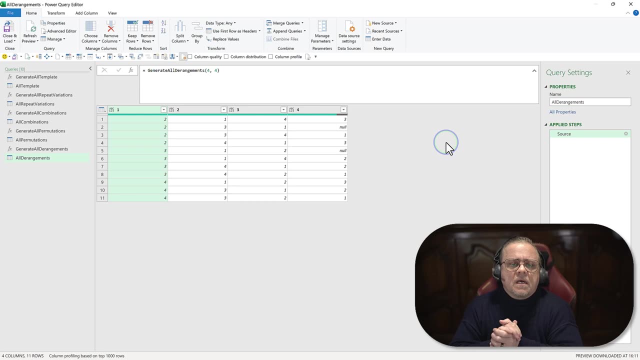 Yeah, but there is a problem. Allow me to show you. We invoke it, give it a good name, all derangements. and yeah, in the fourth column there are nulls, because, well, we've used up all the other numbers in the previous columns and only four could be put here in.